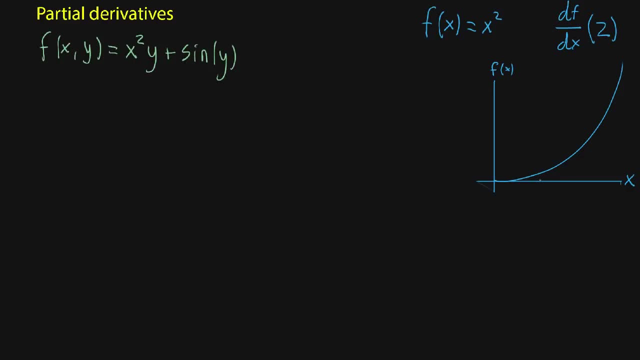 and x squared, has a certain parabolic shape to it, something like that. Then we go to the input: x equals one, two. This little dx here I like to interpret as just a little nudge in the x direction, and it's kinda the size of that nudge. 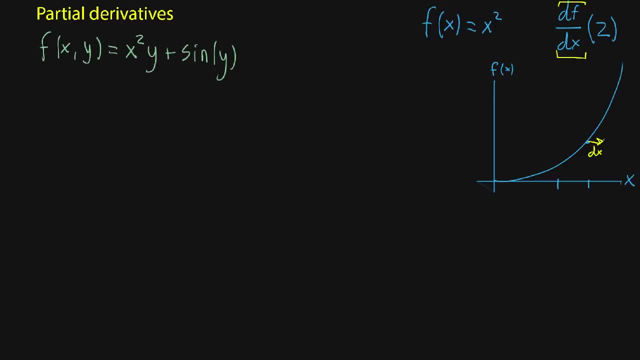 And then df. df is the resulting change in the output after you make that initial little nudge. So it's this resulting change. And when you're thinking in terms of graphs, this is slope. you kind of have this rise over run. 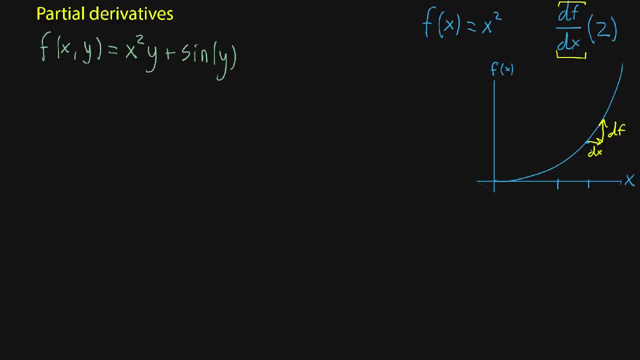 for your ratio between the tiny change of the output that's caused by a tiny change in the input, and of course this is dependent on where you start Over. here we have x equals two, But you could also think about this without graphs. 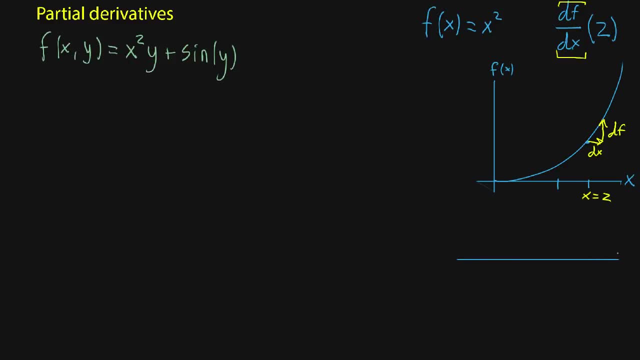 if you really wanted to, You might just think about: you know, your input space is just a number line and your output space also is just a number line, the output of f over here. and really you're just thinking of somehow mapping numbers. 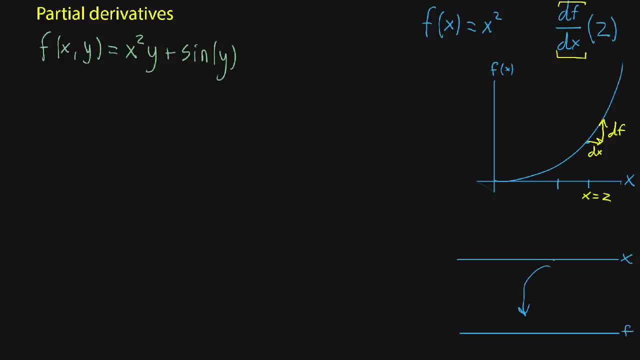 from here onto the second line And in that case your initial nudge, your initial little dx, would be some nudge on that number line and you're wondering how that influences the function itself. So maybe that causes a nudge, that's you know. 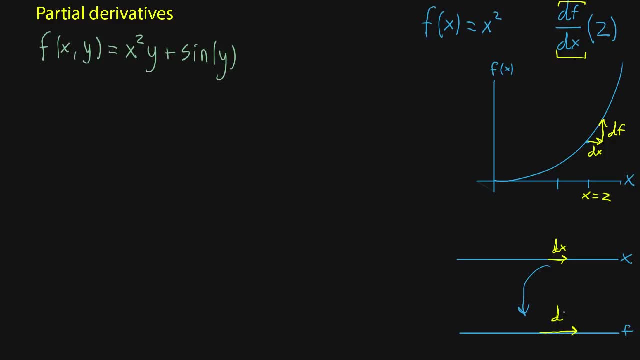 four times as big, and that would mean your derivative is four at that point. So the reason that I'm talking about this is because over in the multivariable world we can pretty much do the same thing. You know you could write df, dx. 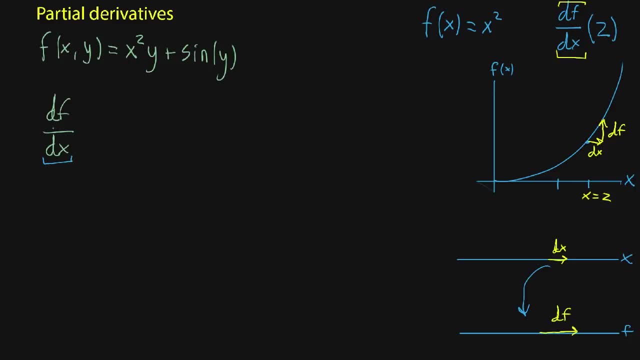 and interpret that as saying: hey, how does a tiny change in the input in the x direction influence the output? But this time, the way that you might visualize it, you'd be thinking of your input space here. I'll draw it down here as the xy plane. 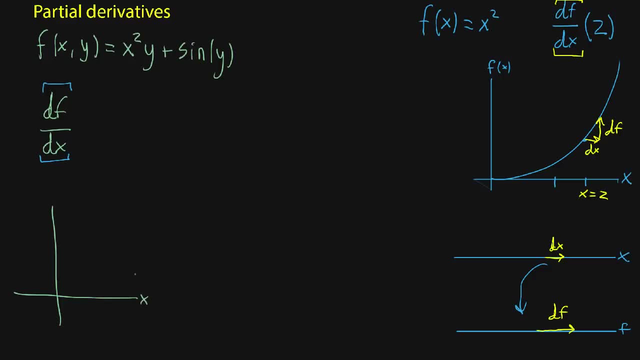 So this time this is not gonna be graphing the function. this is: every point on the plane is an input, And let's say you were evaluating this at a point like one, two, okay In that case, so you'd go over to the input. 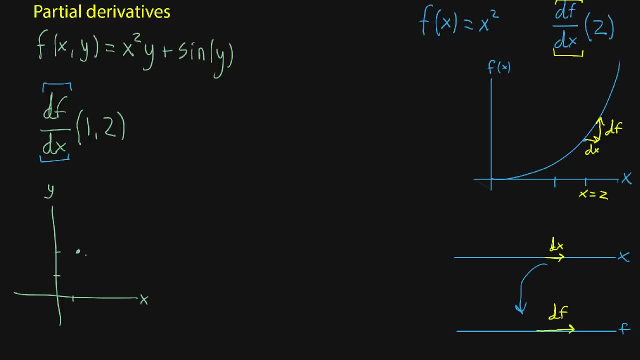 that's one, and then two, and then you'd say: okay, if there's a tiny nudge in the input, this tiny change dx, how does that influence the output? And in this case the output I mean. 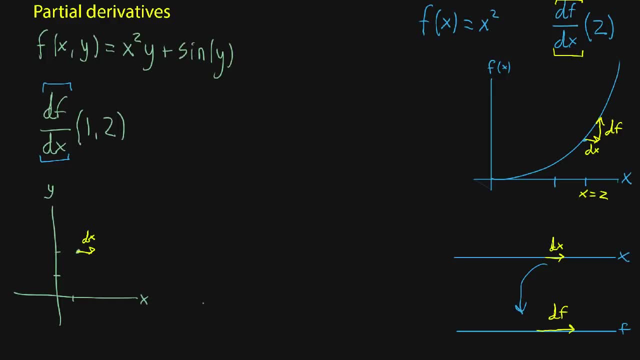 it's still just a number. so maybe we go off to the side here and we draw just like a number line as our output and somehow we're thinking about the function as mapping points on the plane to the number line. So you'd say, okay, that's your dx. 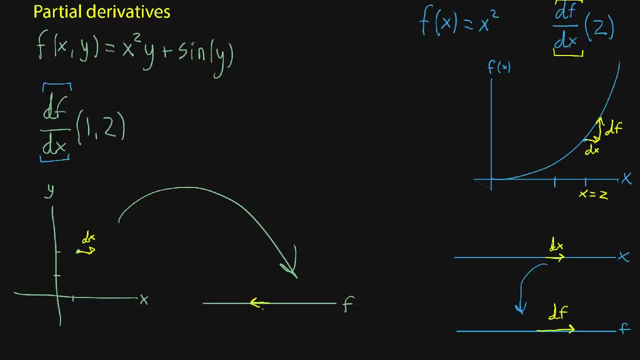 how much does it change the output? And you know, maybe this time it changes it negatively. It depends on your function, Maybe your df, and you can also do this with the y variable, right? There's no reason that you can't say df, dy. 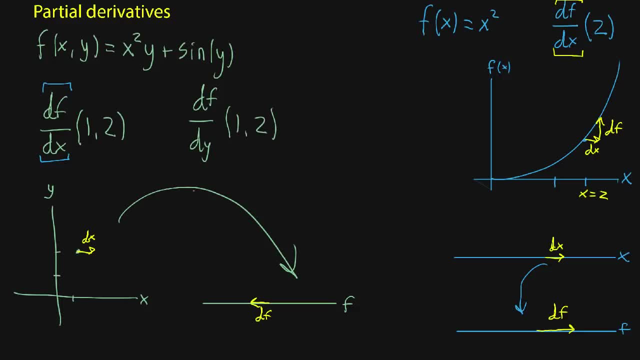 and evaluate at that same point one, two, and interpret totally the same way, Except this time your dy would be a change in the y direction. So maybe I should really emphasize here that that dx, that that dx is a change in the x direction here. 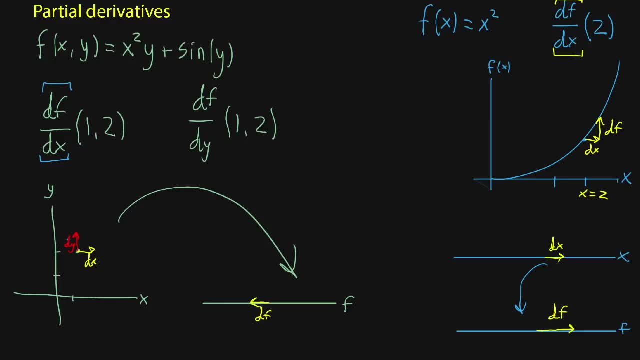 and that dy is a change in the y direction and maybe when you change your f according to y it does something different, right? Maybe you know the output increases and it increases by a lot. It's more sensitive to y. 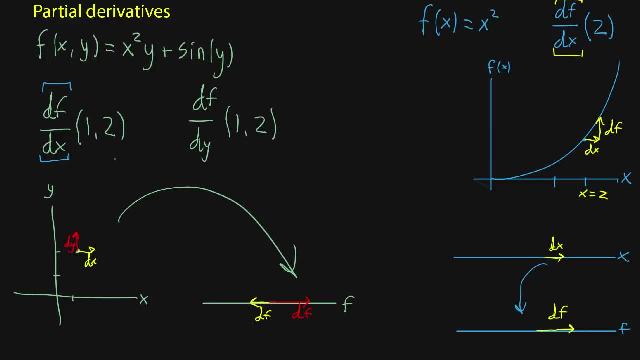 Again, it depends on the function, And I'll show you how you can compute something like this in just a moment here. but first there's kind of an annoying thing associated with partial derivatives, where we don't write them with d's and dx df. 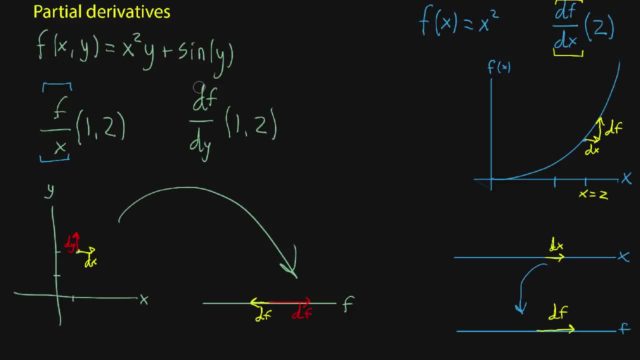 People came up with this new notation mostly just to emphasize to the reader of your equation that it's a multivariable function involved And what you do is you say you write a, d, but it's got kind of a curl at the top. 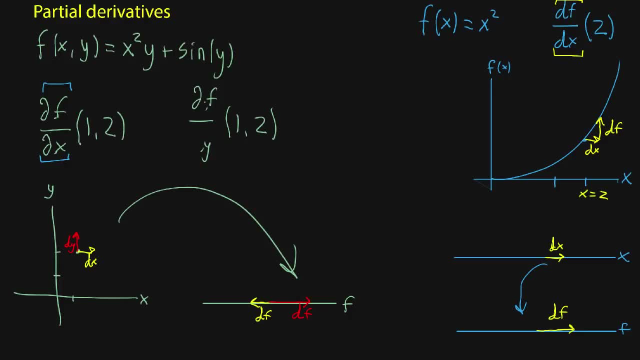 It's this new symbol and people will often read it as partial, so you might read like partial f, partial y. If you're wondering, by the way, why we call these partial derivatives, it's sort of like this doesn't tell. 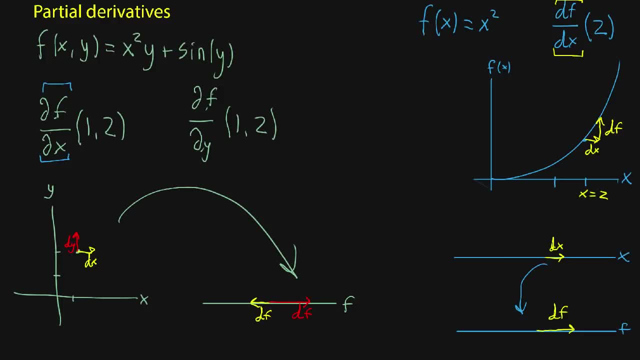 the full story of how f changes, because it only cares about the x direction. neither does this. This only cares about the y direction, so each one is only a small part of the story. So let's actually evaluate something like this. I'm going to go ahead and clear the board. 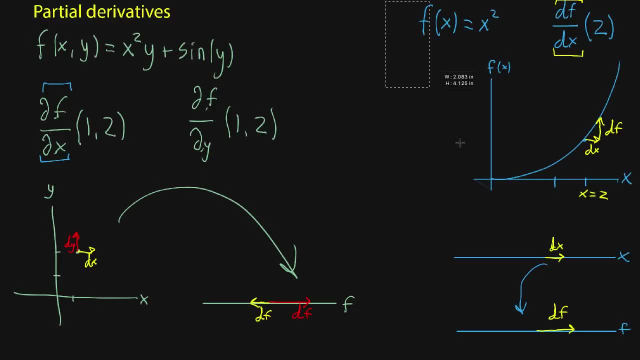 over here. I think the one-dimensional analogy is something we probably have already. So little remnants. So if you're actually evaluating something like this here, I'll write it again up here. partial derivative of f with respect to x, and we're doing it at one two. 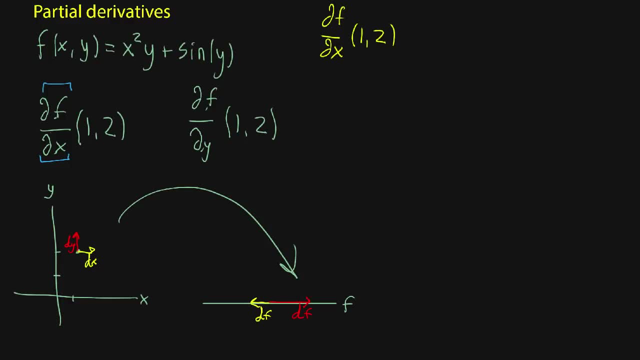 it only cares about movement in the x direction, so it's treating y as a constant. It doesn't even care about the fact that y changes. As far as it's concerned, y is always equal to two, so we can just plug that in ahead of time. 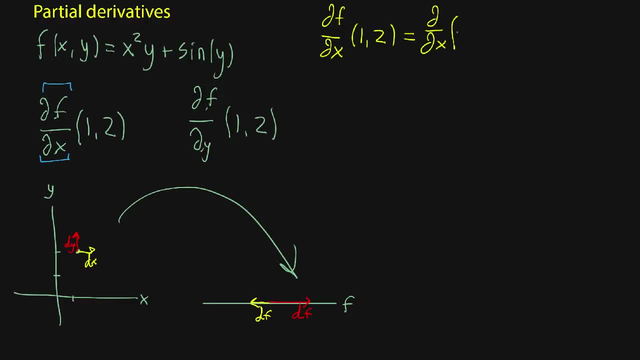 So I'm going to say partial, partial x. this is another way you might write it. put the expression in here and I'll say x, squared, but instead of writing y, I'm just going to plug in that constant ahead of time. 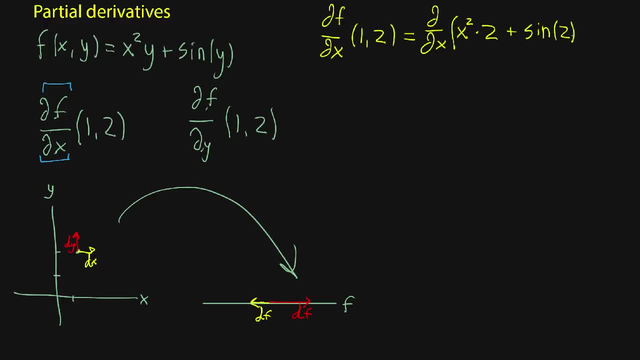 because when you're only moving in the x direction, this is kind of how the multivariable function sees the world, and I'll just keep a little note that we're evaluating this whole thing at x equals one, And here this is actually just an ordinary derivative. 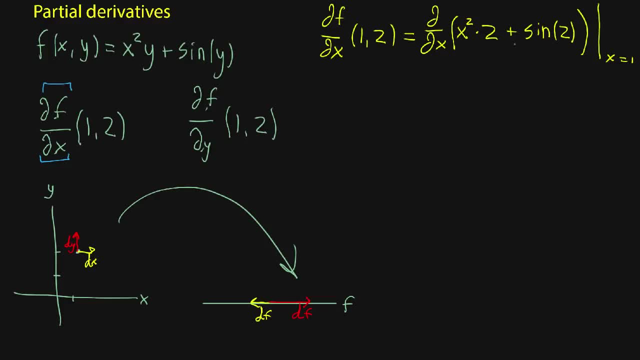 Right, So this is an expression, that's an x. you're asking how it changes as you shift around x, and you know how to do this. This is just taking the derivative. the derivative of x squared times two is going to be four x. 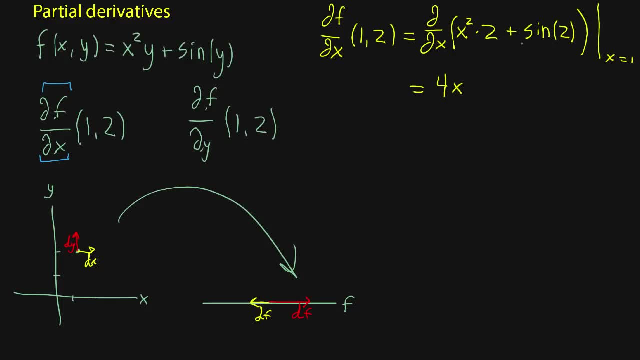 because x squared goes to two x, and then the derivative of a constant sine of two is just a constant is zero, And of course we're evaluating this at x equals one. so your overall answer is going to be four, And just for practice, let's also do that. 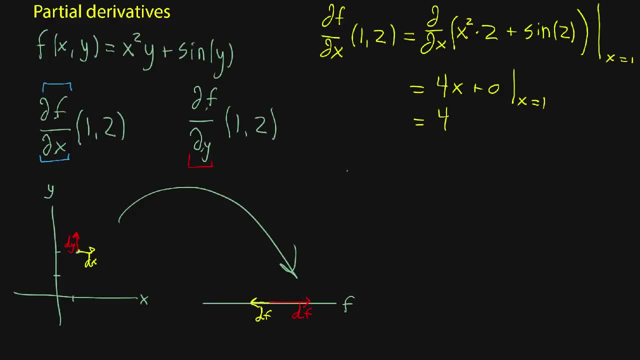 with the derivative with respect to y. So we look over here. I'm going to write the same thing. You're taking the partial derivative of f with respect to y. we're evaluating it at the same point, one, two. This time it doesn't care about movement. 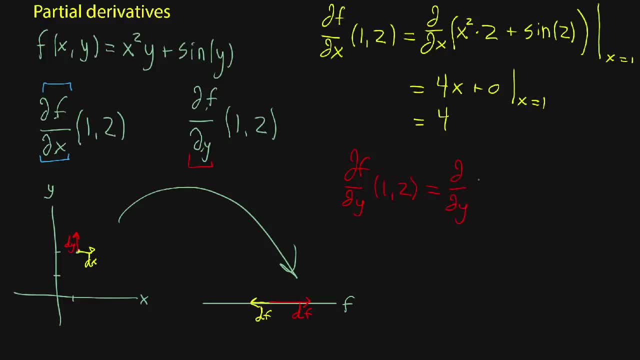 in the x direction. so, as far as it's concerned, that x just stays constant at one, so we'd write one squared times, y plus sine of y, sine of y, and you're saying, oh, I'm keeping track of this. 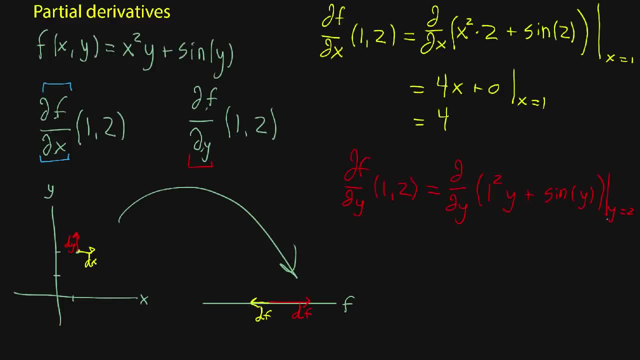 at y equals two. So that's kind of your evaluating. at y equals two, When you take the derivative, this is just one times y, so the derivative is one. This over here the derivative is cosine, cosine of y. Again, we're evaluating this whole thing at y equals two. 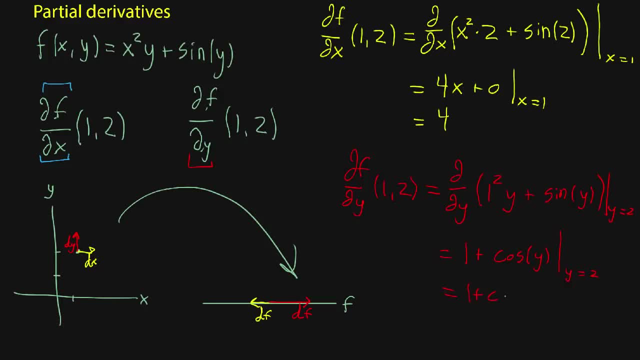 so your overall answer it would be one plus cosine of two. I'm not sure what the value of cosine of two is, off the top of my head, but that would be your answer And this is a partial derivative at a point. but a lot of times you're not asked. 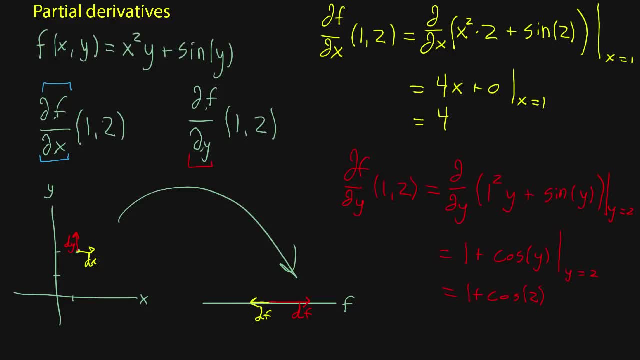 to just compute it at a point. What you want is a general formula that tells you: hey, plug in any point, x, y- and it should spit out the answer. So let me just kind of go over how you would do that. 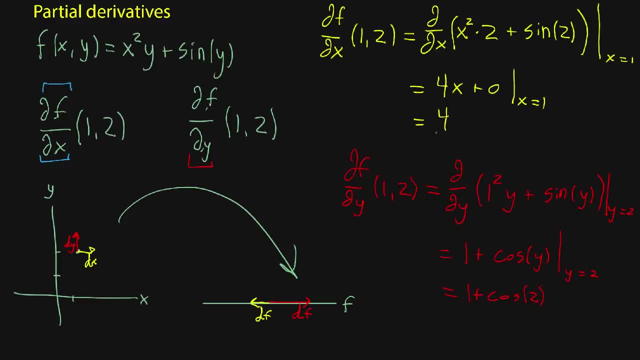 It's actually very similar, but this time, instead of plugging in the constant ahead of time, we just have to pretend that it's a constant. So let me make a little bit of space for ourselves here. Really, I don't need any of this anymore. 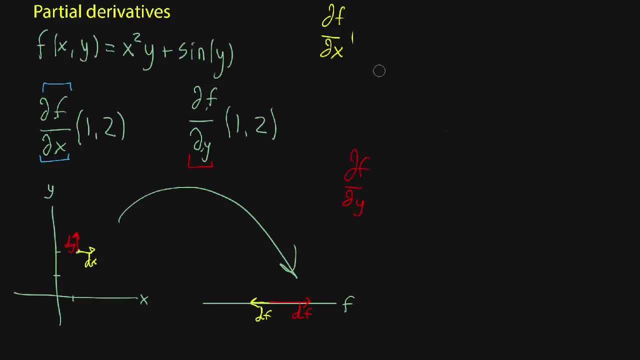 I'm gonna leave the partial partial f, partial partial y. We want this as a more general function of x and y. Well, we kind of do the same thing. We're gonna say that this is derivative with respect to x, and I'm using partials just to kind of emphasize. 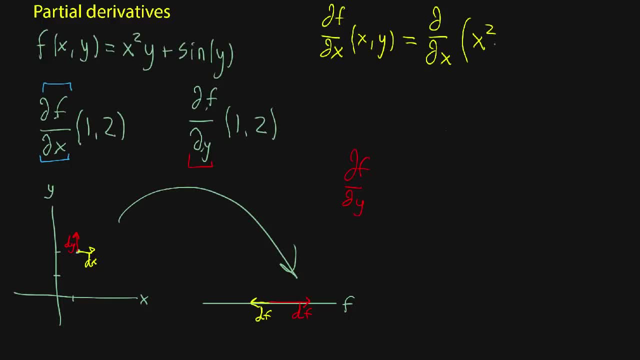 that it's a partial derivative. but now we'd write x squared and then kind of emphasize that it's a constant value of y Plus the sine, and again I'll say y, And here I'm writing the variable y. 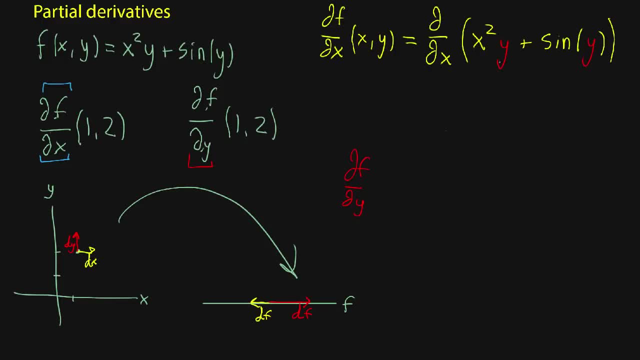 but we have to pretend like it's a constant. You're pretending that you plug in two or something like that and you still just take the derivative. So in this case, the derivative of x squared times a constant is just two x times that constant. 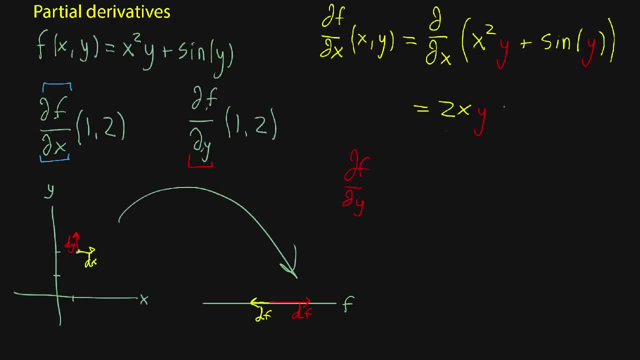 Two x times that constant. And over here the derivative of a constant is always zero, So that's just always gonna be zero. So this is your partial derivative and this is your partial derivative. So this is your partial derivative as a more general formula. 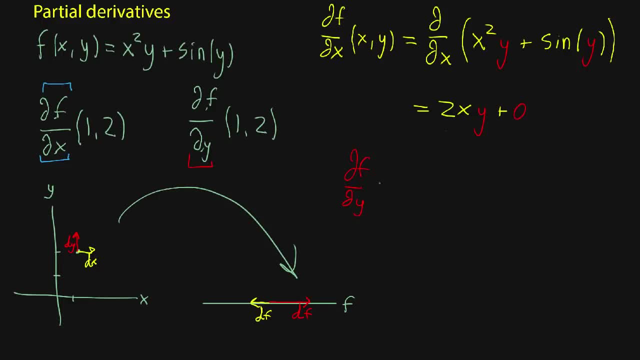 If you plugged in one two to this, you'd get what we had before. And similarly, if you're doing this with f of partial f, partial y, we write down all of the same things. Now you're taking it with respect to y. 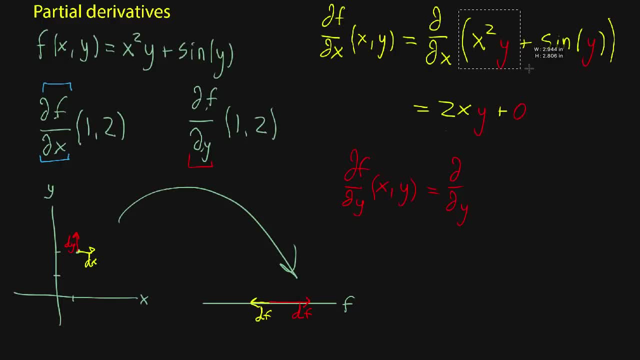 And I'm just gonna copy this formula here. actually, But this time we're considering all of the x's to be constants. So in this case, when you take the derivative with respect to y of some kind of constant, you know, constant squared is a constant.